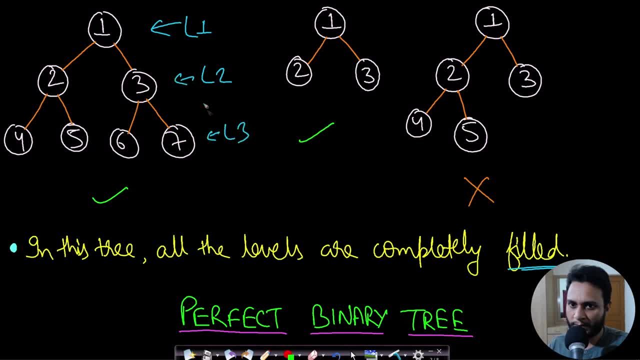 This is level two and this is level three. You can see that at level one, there can be maximum of only one node in a binary tree, So it contains one node. at level two, you can have maximum of two nodes in a binary tree and it is having two nodes at level three. 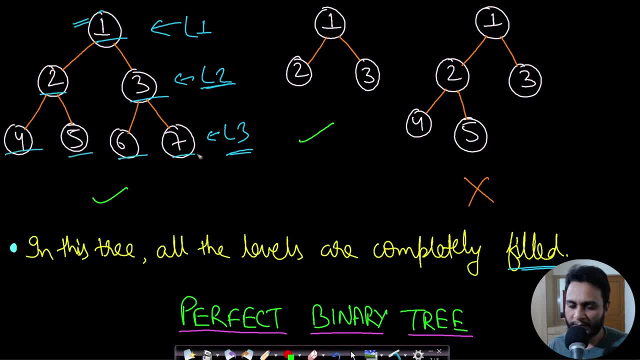 you can have maximum of four nodes in a binary tree and it is having four nodes right, So all the left and right childs are filled. That means if the depth is, let's say, n, then up till level n minus one, All these will be the internal nodes, So all the leaves will be lying at the nth level. 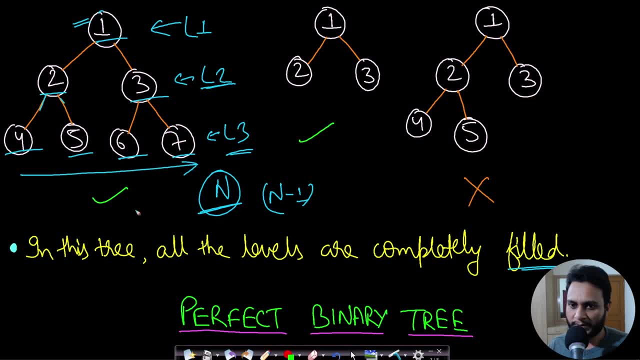 that is at the last level, and all the leaves will be present, right? So this is what perfect binary tree means. Now, in the second case as well, this is also a perfect binary tree, because this is level one. it should have maximum of one node. here, one node is contained. 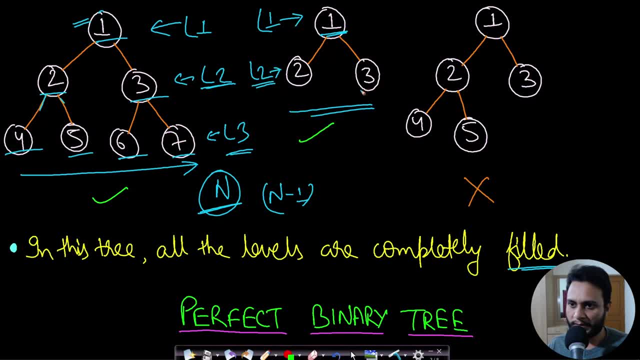 at level two, maximum should be two nodes, and two nodes are contained. There is no other level. Okay, so that is why this is a perfect binary tree. In the third case, you will see that This first level should contain maximum of one node. So this is containing one node, right? 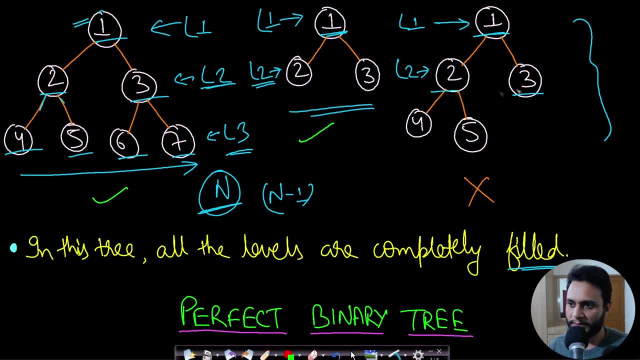 Second level should contain two nodes, which is maximum. So this is containing two nodes, But then when you come to level three, it should contain four nodes, because this is maximum. okay, maximum which can be kept at level three should be four nodes, But in this, 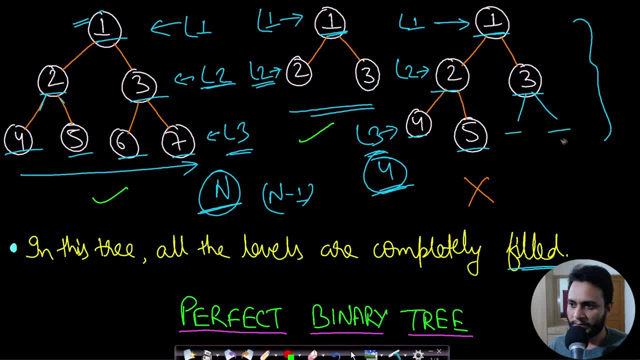 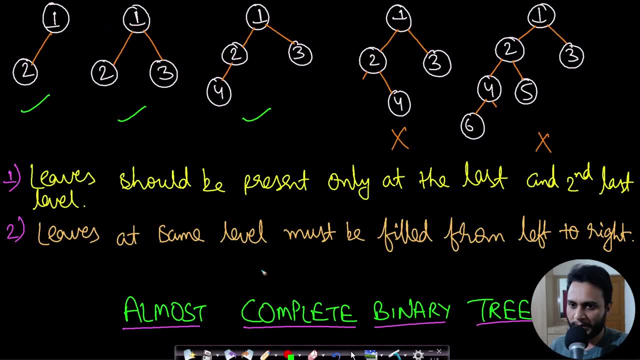 case, there are two nodes here. you can accommodate two more nodes, So these are not present, and that is why this is not a perfect binary tree. I hope you understood the concept of perfect boundary tree. Let's now move on to the almost complete binary tree. What does this mean? 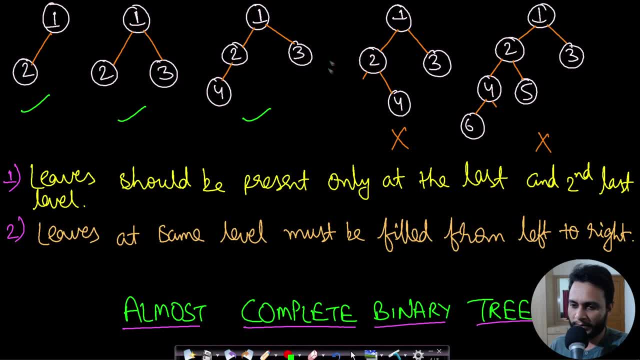 An almost complete binary tree will never be a perfect tree. okay, that means a perfect binary tree. So in this case, the leaves should be present only at the last and the second last level, And the leaves at the same level must be filled from left to right. Now let's. 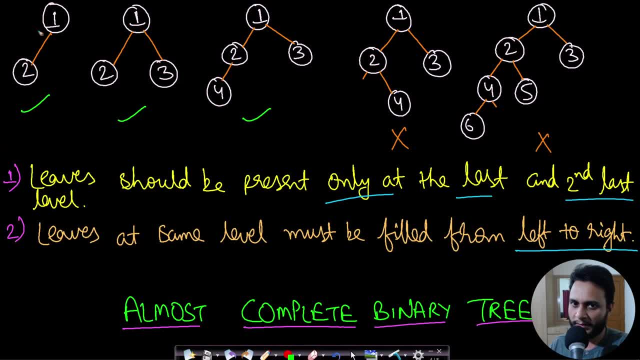 see some examples. In the first example, you will see that this is the second last level. okay, Because the depth is too. the second last level will be depth one, which is this one l1 level. okay, so till l1 level, the tree is entirely filled. okay, at the last level, the tree should be filled from left to right, and this is 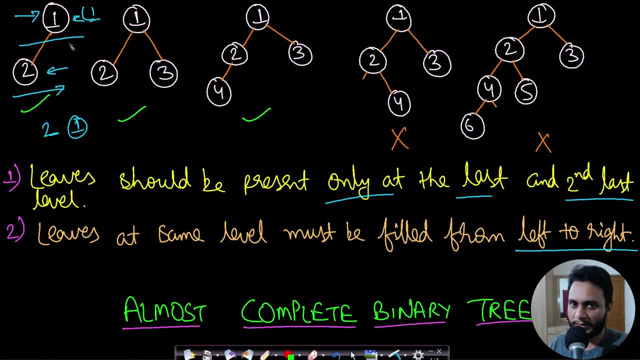 correct, because if two would have been the right side of this one, then this would not have been an almost complete boundary, but since two is the left side of one, so we are following, the property that leaves at the same level must be filled from left to right. okay, now in the second example you will 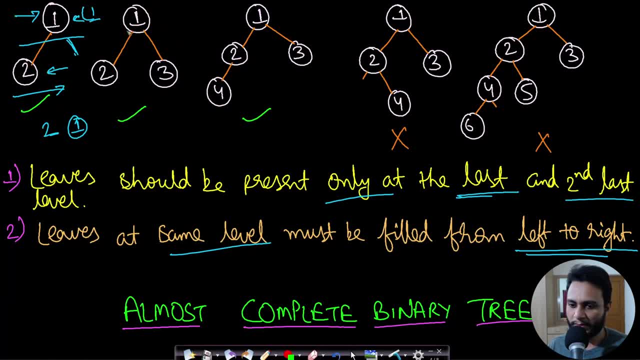 see that this is a perfect boundary tree. this is not a almost complete boundary, so this is not an almost complete boundary. in this case, level one is completely filled, as well as level two is completely filled, so this will be a perfect boundary. this is not almost complete boundary. 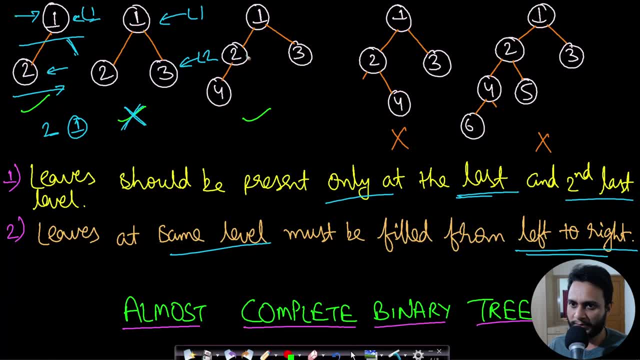 in the third case, this will be an almost complete boundary tree. why is that? because this first level is filled. the second level is intact filled. this is the n minus 1th level. now this is the last level. at the last level, all the nodes should not be present, but the nodes should be present from left to right. okay, so in this case, 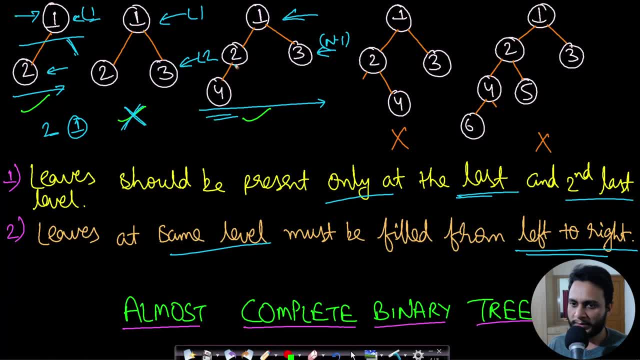 if 4 would have been present. if there is only one node, then that should have been present. as a left side of 2, let's say there was another node here, 5. okay, so will this be an almost complete binary tree? no, because if 5 is present, then this should be present here, because we want to fill from left. 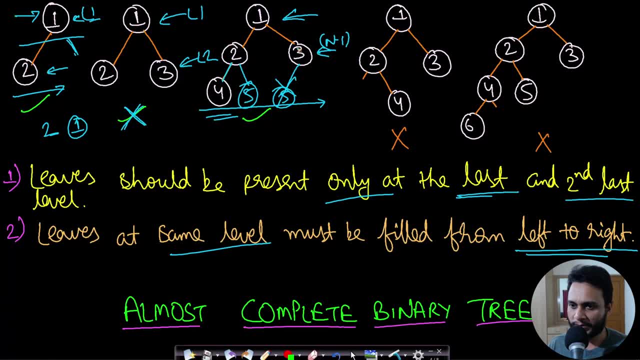 to right and this should be removed. then this will become a almost complete binary tree. i hope you are understanding it now in this example. in the fourth example you will see that this is not an almost complete binary tree because first level is filled, second level is filled, all right, but in 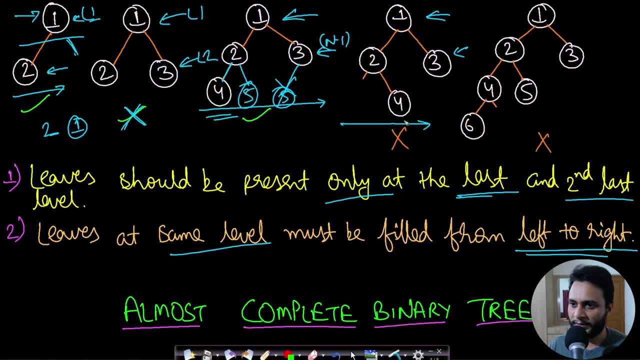 the last level, leaves should be filled from left to right, but here you will see that 2's right child is 4, but left child is not present. so this rule is not being followed. this second rule: now, in this last example we will see that this is: 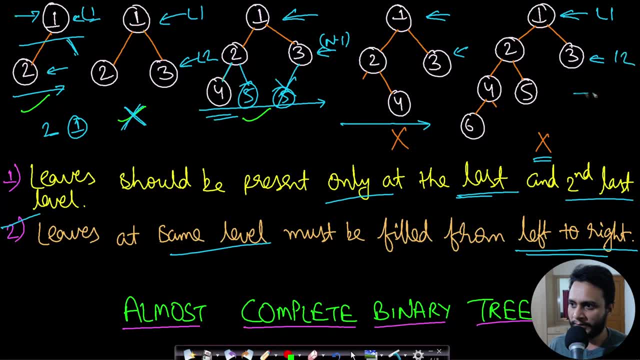 complete binary tree and this should be removed. then this will become a almost complete binary tree, filled L1 level. L2 level is completely filled. L3 level is not completely filled. So the first rule says that leaves should be present only at the last and the second last. 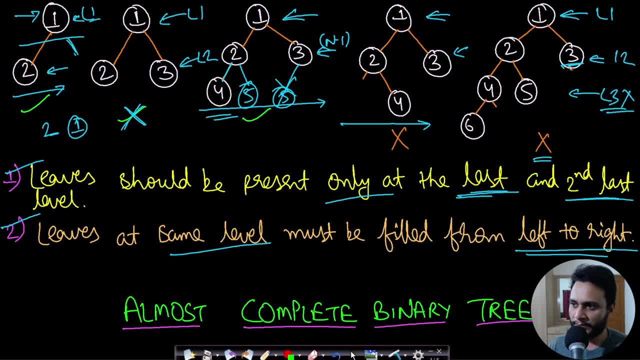 level, But you will see that this is this. three is a leaf, Okay, And this is present at the third last level. This is level three. This is level four. Okay, So this is the last level and this is the second last level. So what is this L2 doing? This is the third last level and this is. 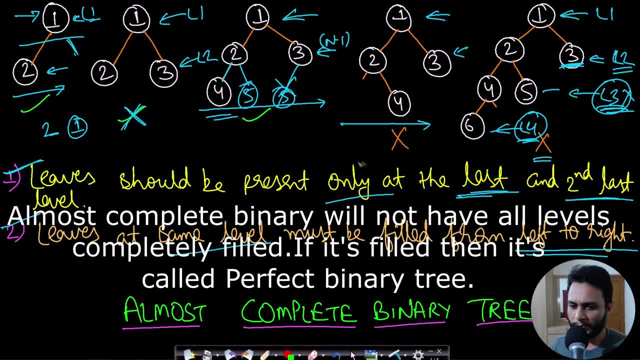 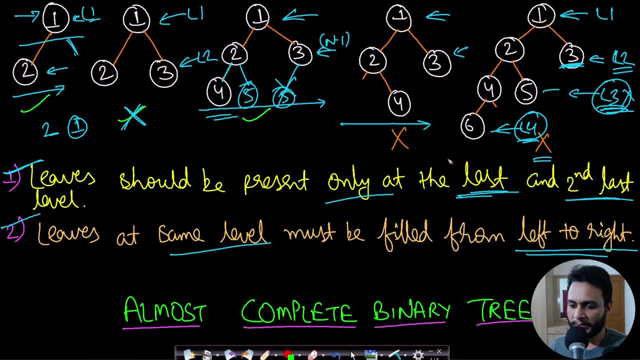 leaf. so this first rule is not getting followed. so i hope you understood both the perfect binary tree as well as almost complete binary tree, right? so if you just google it out, then basically you might get confused. so just follow the video, so now you will quickly understand what is a complete. 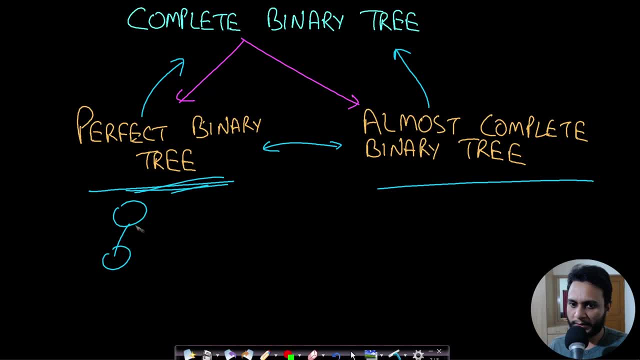 binary tree. now, a perfect binary tree should contain all the levels, completely okay. so if it is having two levels, it should have three nodes. if it is having three levels, then it should have seven nodes, right? so this is a perfect boundary, and an almost complete binary tree should not be. 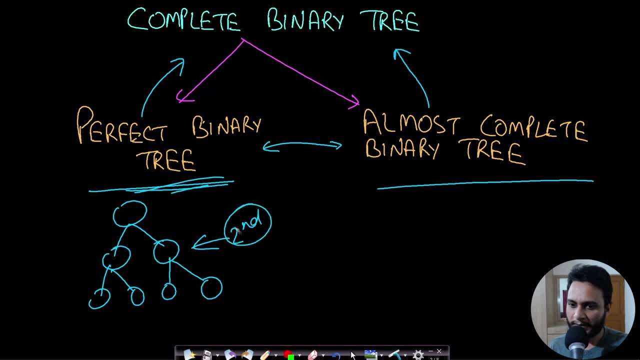 perfect. second last level. until the second last level, everything should be full right, and at the last level if we are filling nodes, then that should be present from left to right. so this is an almost complete boundary. so what can we say about this complete boundary tree? we can say that 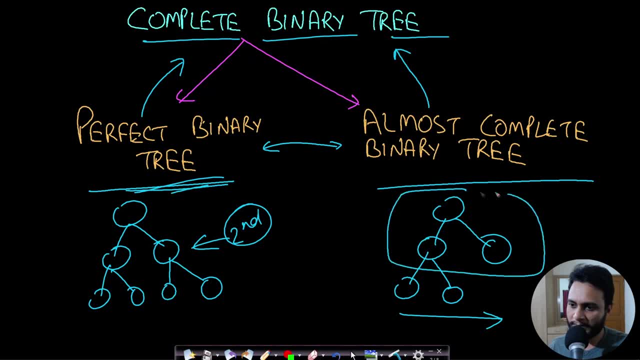 in a complete boundary tree. all the levels till the second last level- second last level- is completely filled, right, but at the last level the nodes should be filled from left to right. okay, and all the nodes might be present, okay. so this is also a complete boundary. this is not an almost complete boundary, it is a. 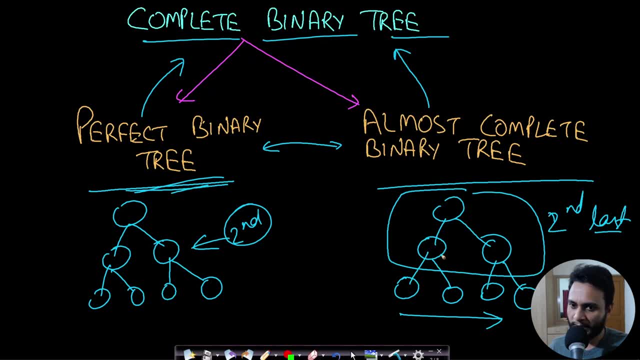 complete boundary tree and this is also a perfect boundary right. so basically, this is very simple to understand. if you are having a tree, then until the second last level, all the levels should be completely filled. at the last level, the node should be filled from left to right. that's it okay. 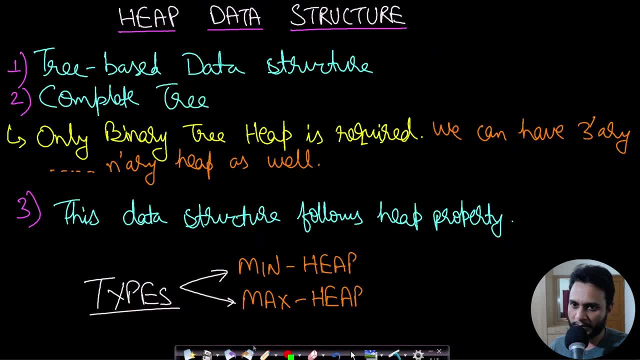 so i hope you understood this concept as well. now, once you have understood this, let us look at what a heap data structure really is. in this case, a heap data structure is a tree based data structure, and it is a complete tree. okay, so a heap can be a binary tree or an anery heap as well, but, uh, entry heaps are not. 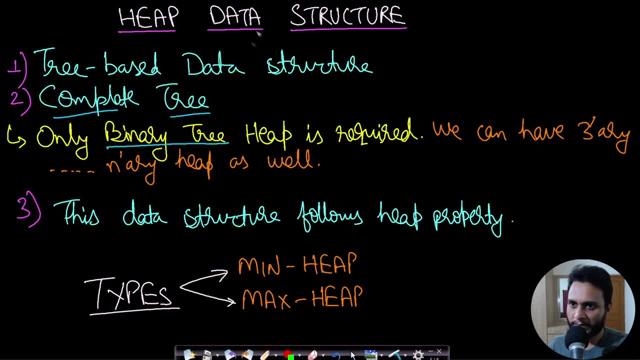 required in this case. we will just be focusing on the binary tree. so what is a heap data structure? now, it should be a complete binary tree. okay, and this is a tree based data structure. third point is that heap property must be followed by this tree based data structure, which is: 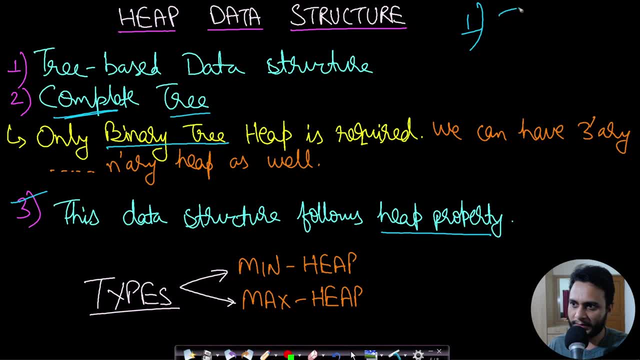 a complete binary tree, okay. so first thing is that this is a tree ds. second thing is that it is a complete binary tree, okay. and the third thing is that it should follow the heap property. so these are the three things which you should remember. so now we will look at the heap property by using examples. so heap is of two types. 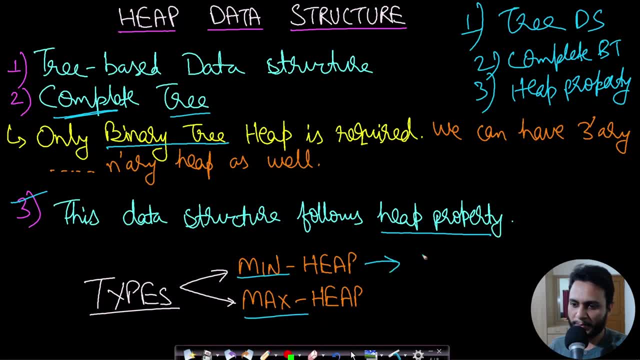 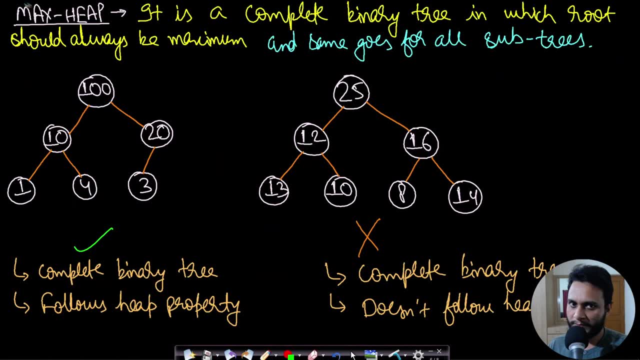 min heap and max heap. min heap keep tracks of the minimum element at the root node. max heap keep tracks of the maximum element at the root node. okay, so now let's first understand what a max heap is. it is a complete binary tree in which root should always be maximum. 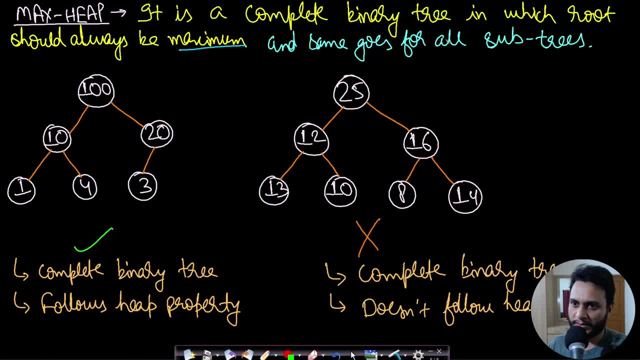 and the same goes for all the subtrees. now, what does this mean? let's look at the first example. in this case, is this a max heap? now you can see that this is a root node, right? so this root node should be maximum in this entire tree, and this is correct. now we need to verify for all the 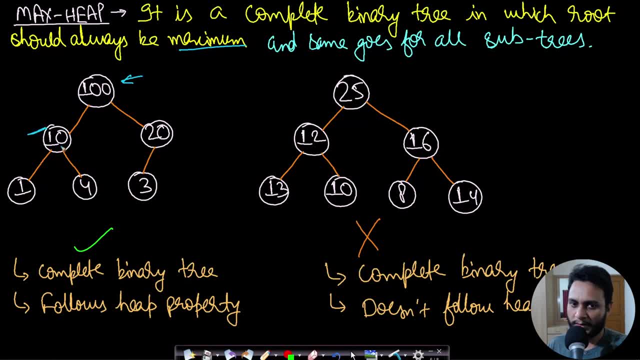 other nodes as well. so if we pick this node 10, then this node 10 is present as a root in this subtree right, and this 10 is greater than both the left subtree as well as right subtree. that means all the elements in left subtree and all the elements on the right. 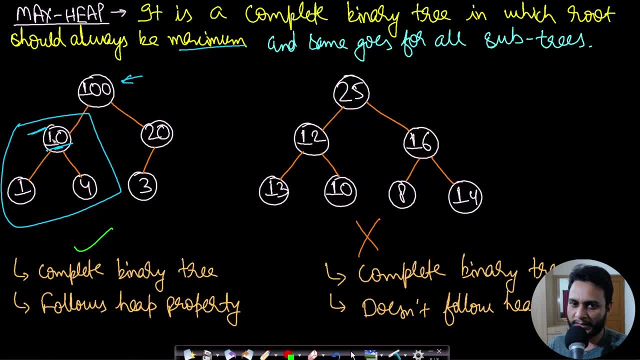 subtree. if you combine them, then this: So this is the maximum element. okay, this is what a max heap property means. now, in this case, if you look at this 20, then in this subtree, 20 is the root node and in this entire subtree, 20 is the maximum element. okay, so this is what a max heap property means. it means that 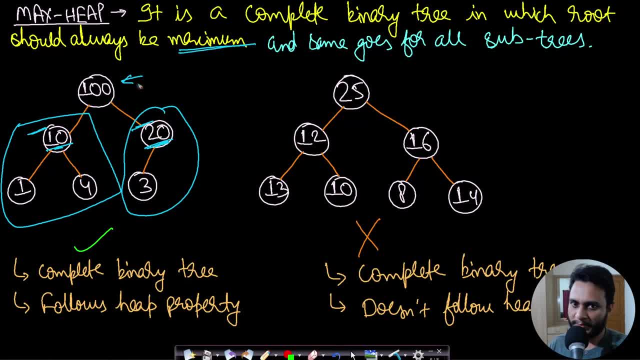 the root should always be maximum and the same is followed recursively for all the subtrees. okay, look at the second example and understand if it is a max heap. so if you look at the second example, then this is the root, node right, and this is the maximum in this entire tree. okay, so the heap 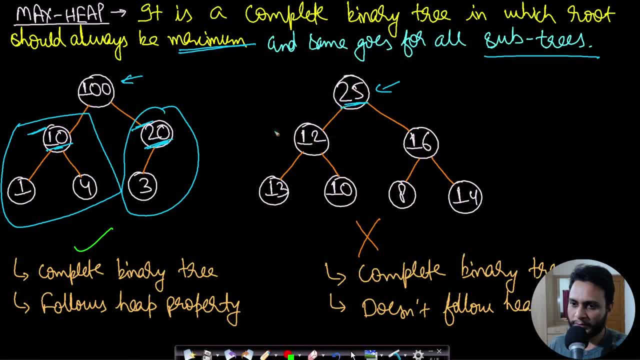 property is being followed for this node. now we will have to check for all the internal nodes recursively, right? so in this subtree 12 is the root. now 12 is the root. so 12 should be the maximum element. but you will see that there is a node in the left subtree which is having higher. 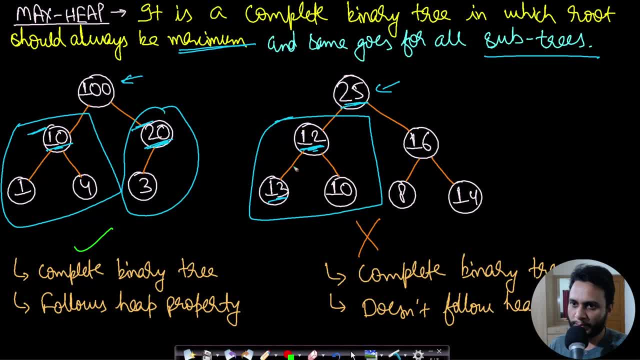 value than this 12.. so this is not following the heap property, right, because the root should always be maximum, even for the subtrees. so this will not be a heap. okay, so both these are complete binary trees, but in the first case it follows the heap property. in the second case it will not be. 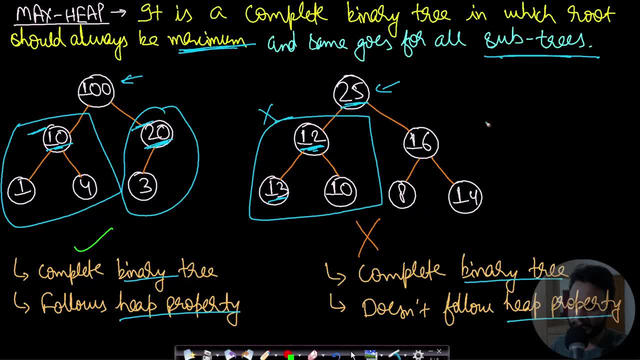 following the heat property. so that is why the second case is not a heap. i hope you understood this map and if you have any questions, please feel free to ask me in the comment section below. so that is why the second case is not a heap. i hope you understood this map and if you have any, 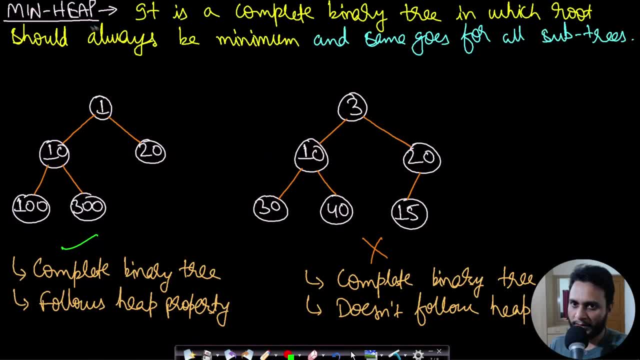 questions please feel free to ask me in the comment section below. now the same goes for the min heap. in a min heap it is a complete binary tree in which root should always be minimum, and the same goes for all the subtrees, right? so this is basically the same concept as the max heap, but in this case the root should. 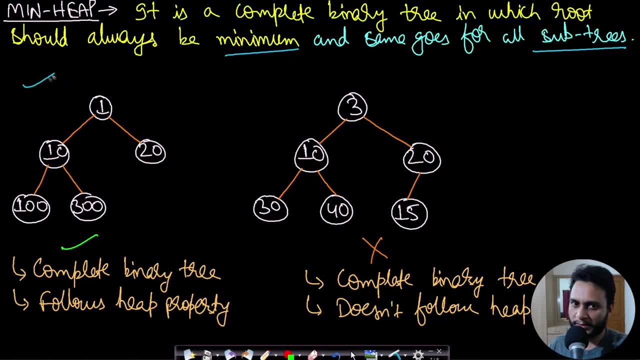 be minimum and in the max heap it should be maximum. so let us quickly look at this first example. in this case, this is the root, so this is having value one. now this should be the minimum value in this entire tree and this is correct right now. we need to verify. 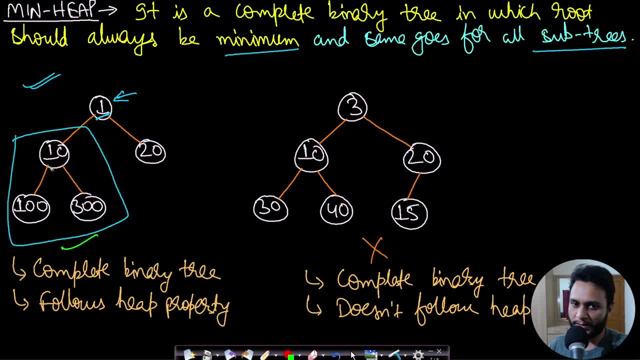 for all the other internal nodes. so if you look at this subtree here, the value is 10 and this is minimum in this entire subtree, right? so this internal node has been verified. now this is a leaf node, so this will not be verified. so the heap property is getting followed for all the internal. 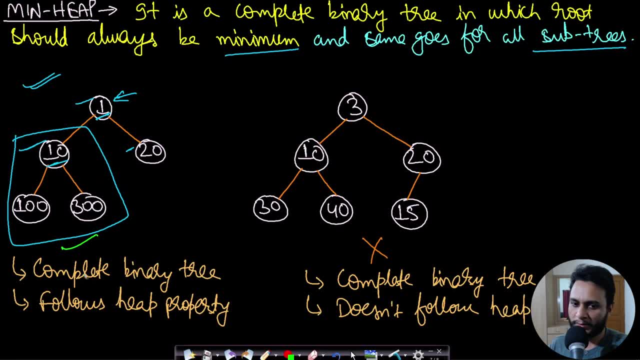 nodes, and that is why this will become a mean heap. so this is a complete binary tree and it follows the heap property. okay, now in the second example, if you look at it, is it a min heap? well, no, it is not a min heap. so how is that? if you look at this root node, this is three and this is minimum in. 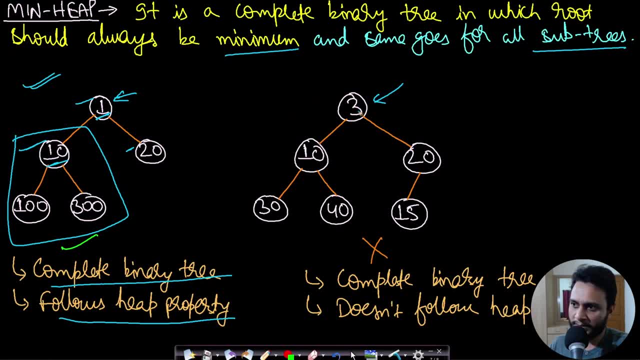 this entire tree. so the min heap property is getting followed here, right. so we will have to check for all the other internal nodes. 10 is an internal node and in this case, uh, you will see that in this subtree, 10 should be minimum. so, yes, it is correct, 10 is minimum, so mean heap property.